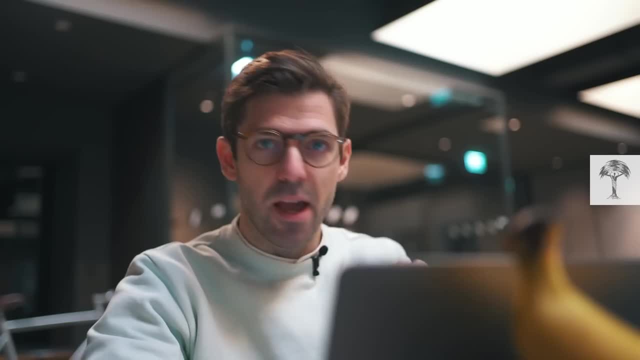 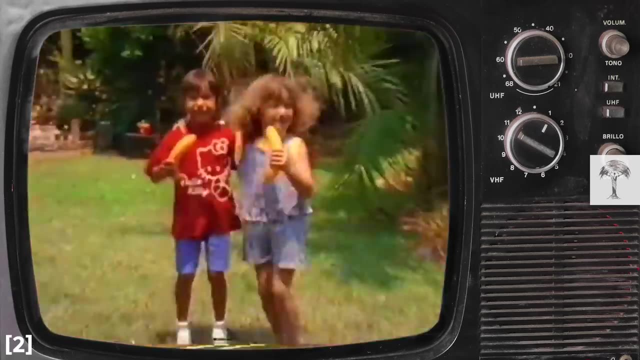 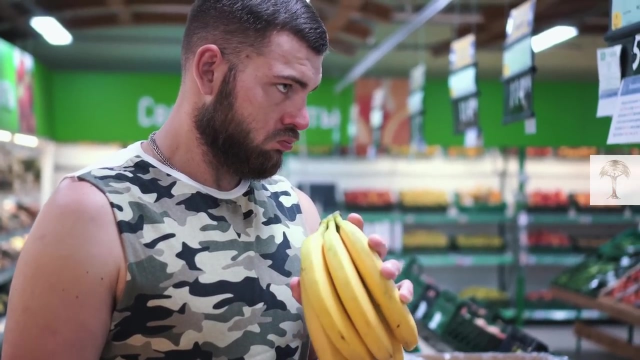 of course, the banana. This, at least for me, has always been like that. Bananas were always there, the perfect complement to activities or sport, a quick way of satisfying hunger or for fancy occasions, slurped as a milkshake. Few people ever really put much thought into it To most of us. 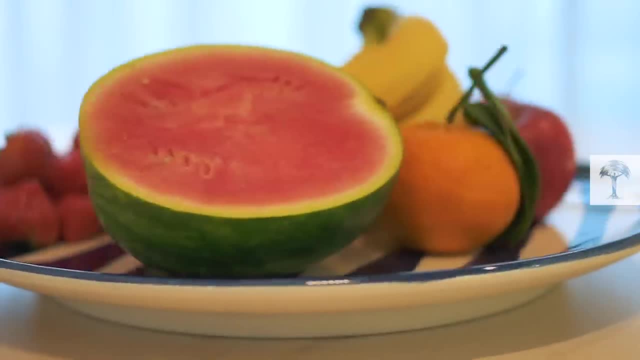 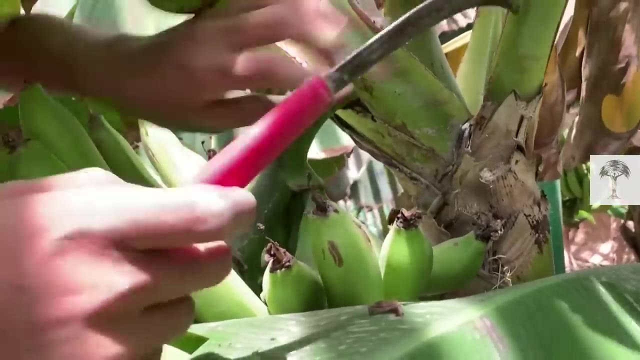 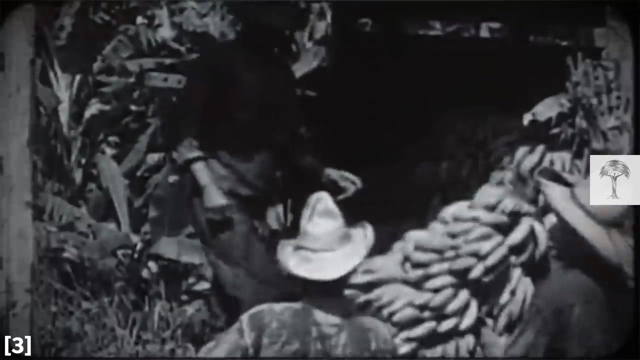 the banana is a simple yellow, tasty, yes, but not at all extraordinary fruit. But what if I told you that I'm pretty sure you and I have eaten a banana picked from the exact same tree? Yes, correct, Not species or kind: the exact same plant. And this one tree has turned the world. 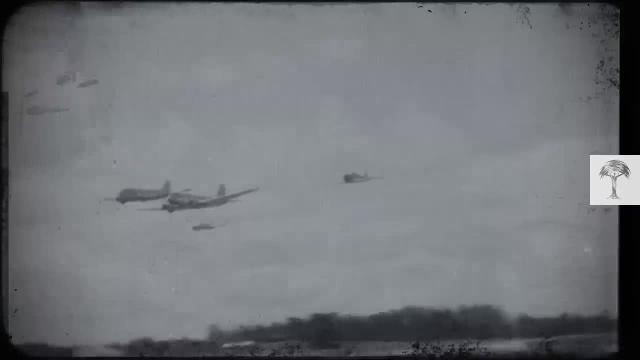 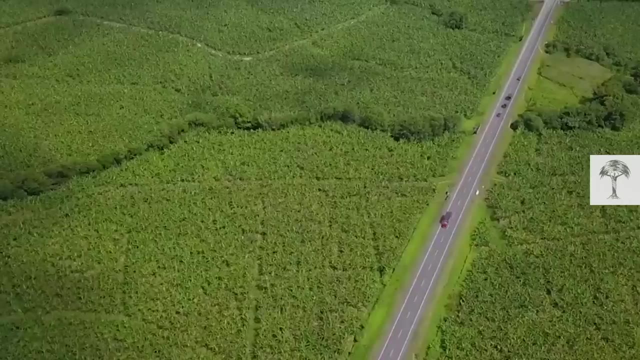 agriculture upside down, being used as a weapon to overthrow entire countries and perfected the trade and value chains of the global food industry, from the fields in Costa Rica or Malaysia to your next supermarket. But now a tiny little fungus known as the Panama disease means that this. 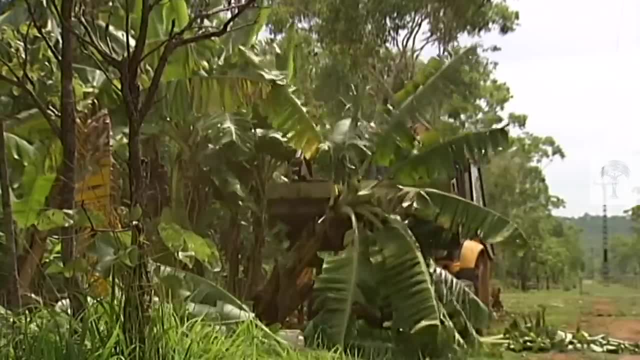 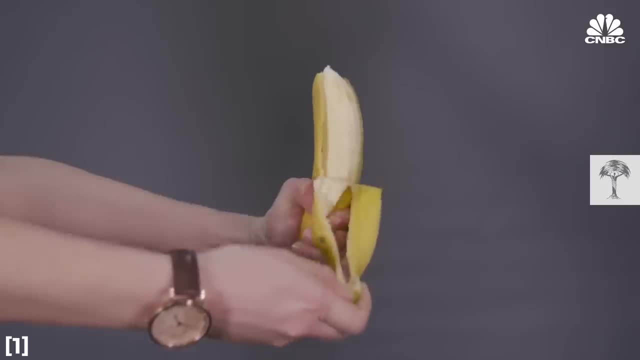 billion-dollar industry could collapse. The banana would suddenly disappear out of our lives, And I know Vice Tony Harris, CNBC and many other channels have already covered this topic. But what's even more fascinating is what we actually do, What we actually can do about it, The way to rescue the fruit, if this is what we want. 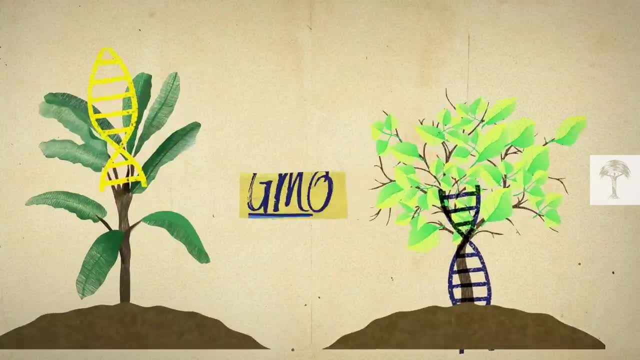 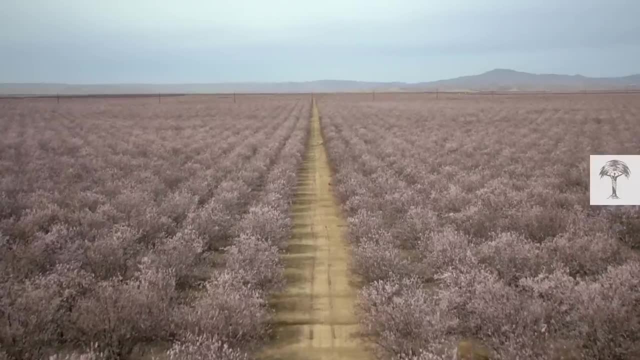 might be through genetic modification. As such, the banana could be our way out of a totally messed up agricultural system that needs complete reboot. Why? Because we have to make our crops fit for future threats and needs. The fate of the banana is a story about something much bigger. 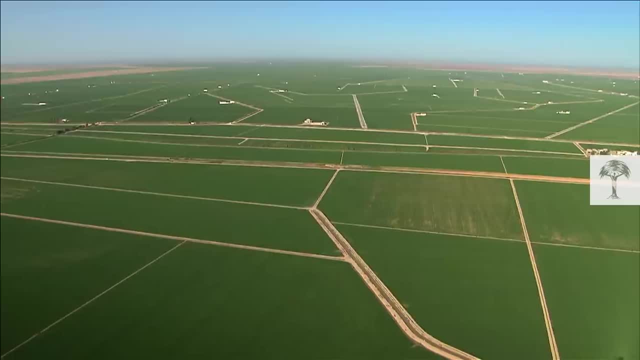 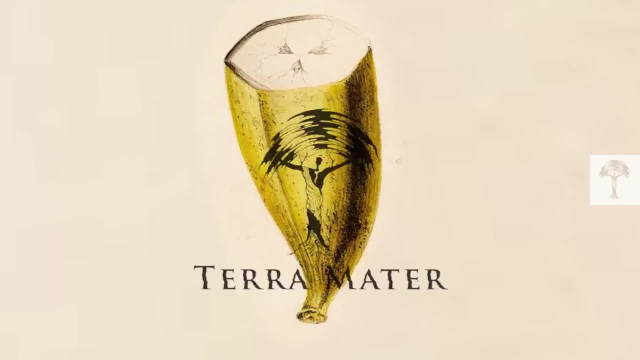 It's about monocultures and the decaying of the richness of our planet. It's the question whether we can or want to do something about it, and whether we are bold enough to rethink the system. The banana truly is an outstanding fruit. Its history is deeply connected with ours. 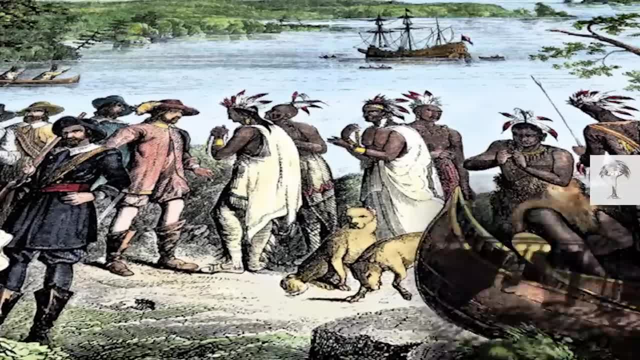 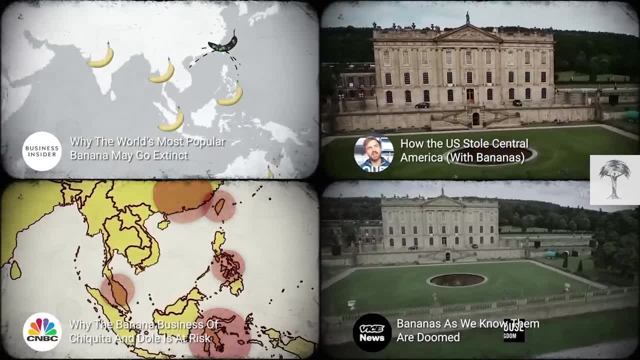 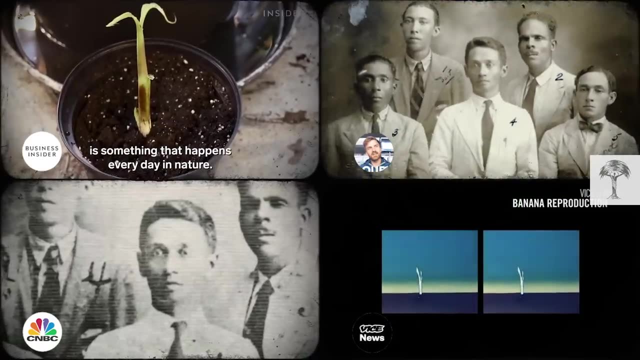 from the beginnings of sedentism to worldwide exportation, trade and colonialism. So short disclaimer at this point. Many fascinating stories around the banana, from coup d'etats in Central America to the providence of Banana Republic and the current crisis the global industry faces due to the Panama disease, have been covered by 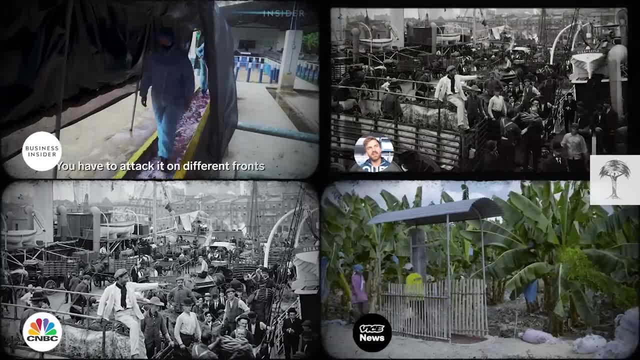 the usual suspects on our most favorite YouTube channels. in a more or less similar way, At some point in time, we will be able to find out more about the banana, and we will be able to find out how. it's even strikingly similar. The links are posted below, so if you haven't seen them, go ahead and have a look. 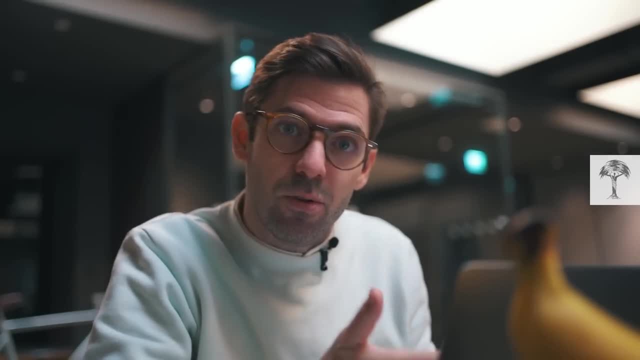 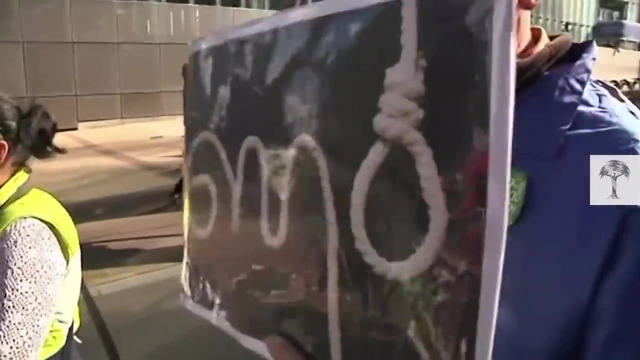 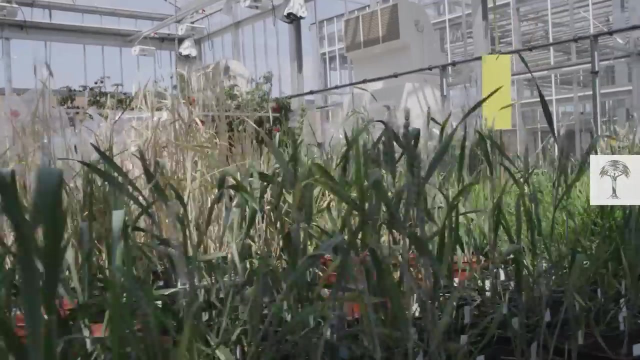 But what staggered me the most- and this is something those channels paid little attention to- is that the solution to save the banana is actually out there. What's preventing us from implementing this theoretically oven-ready solution opens up a much more fundamental yet vital discussion. The future of Europe requires innovative action Through centuries of perfecting. 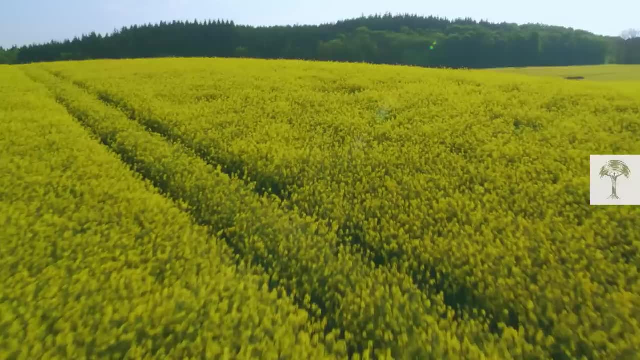 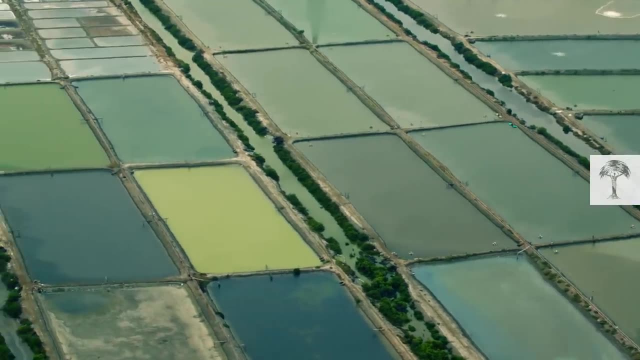 and maximizing agriculture, we've maneuvered ourselves into a situation where our crops in general are not only a source of harm to biodiversity, but also a source of harm to the population diversity and a threat to our planet, but also extremely susceptible to new challenges. 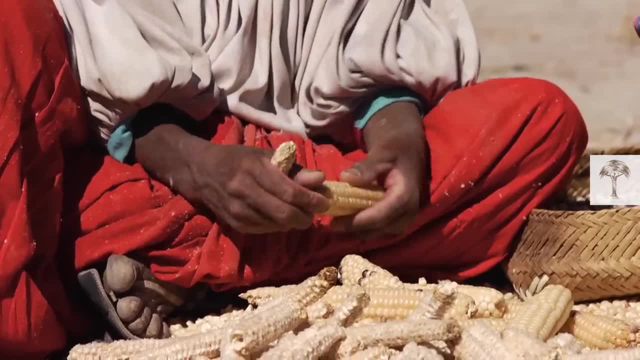 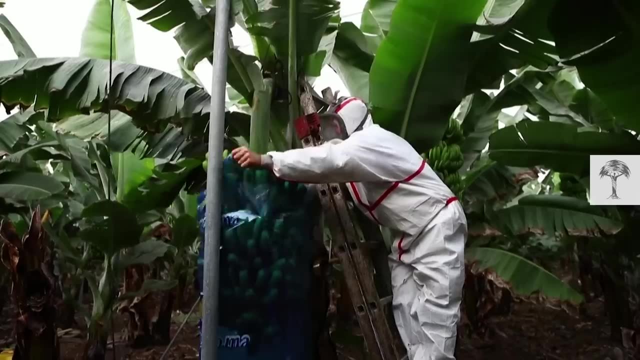 such as draws or diseases. And while wheat and corn might be the father and mother of global monocultures, the banana is a wonderkind And now, with little time left to save the food, the question is whether the way out of this mess really is genetic modification, and how. 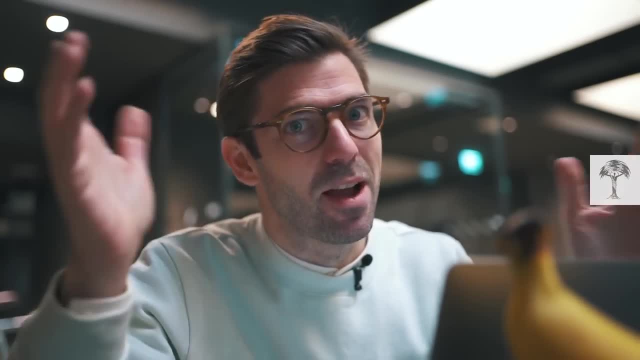 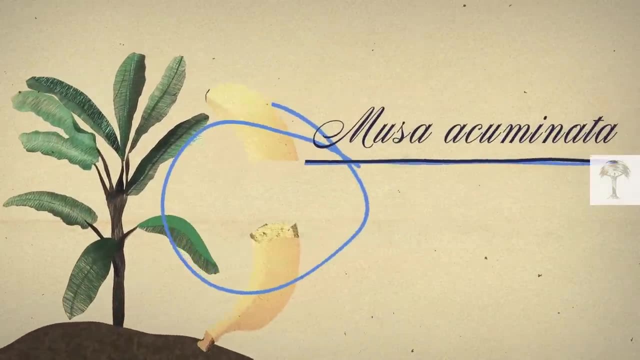 To understand this issue much better. I figured that a crash course in bananology might come in handy. This is the banana that most of us are familiar with: the Cavendish, or Musa Acuminata, as the species is scientifically called. 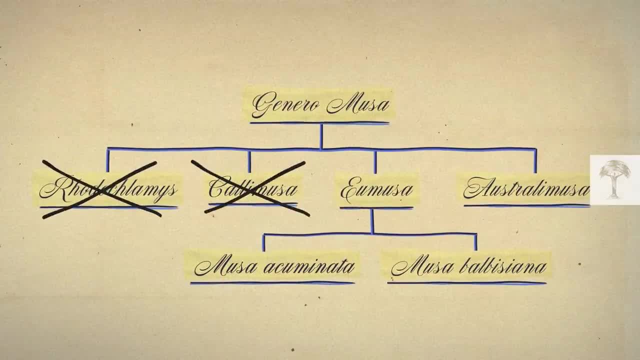 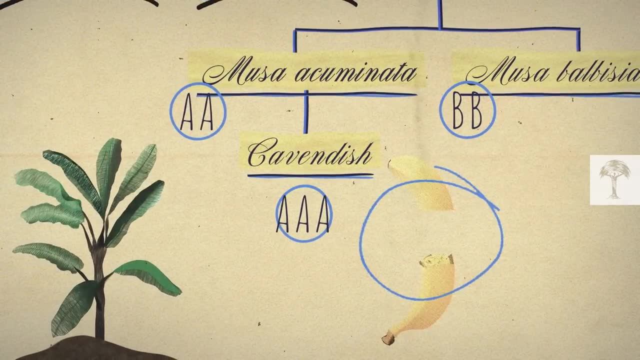 There are four types of Musa, of which only two are edible for humans, and these contain a different combination of A and B genes. The Cavendish is a triple-A hybrid, a combination indicating that it isn't found in the wild. 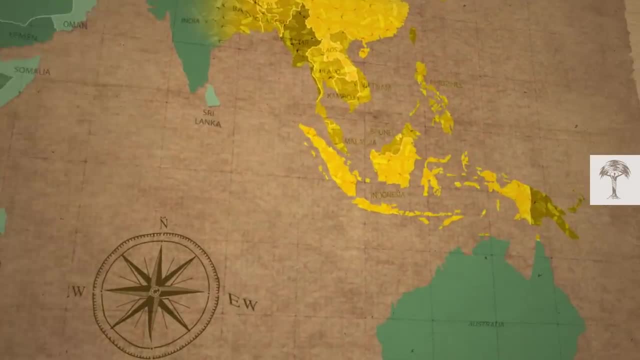 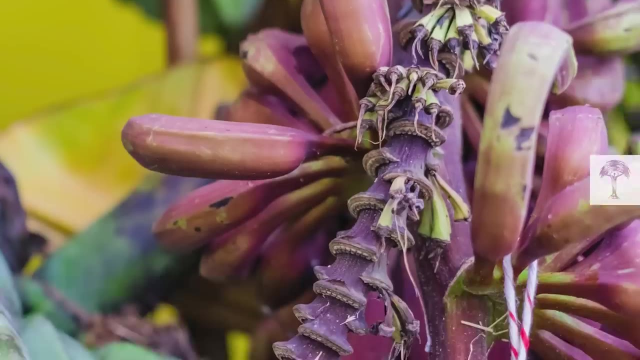 The banana originates in Southeast Asia, where its wild relatives grow in all different types, shapes and forms. from the deep jungle all the way up to the Himalayas, You can find green, brown, orange or even blue bananas. Some can be eaten raw, others are meant to be cooked. 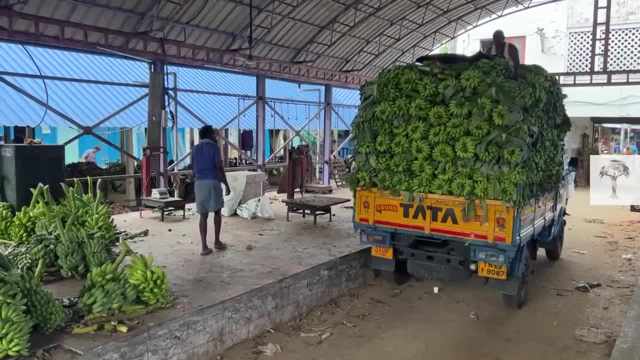 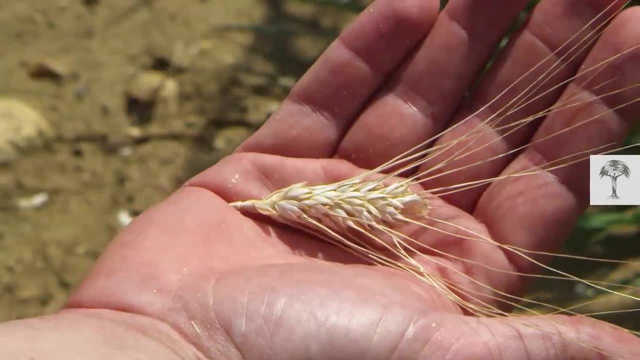 And India is the banana capital, where roughly 700 different types. But when humans became sedentary, we started domesticating the fruit alongside other crops, breeding it to accommodate our needs. Thousands of years of agriculture narrowed the number of bananas down to only a few. 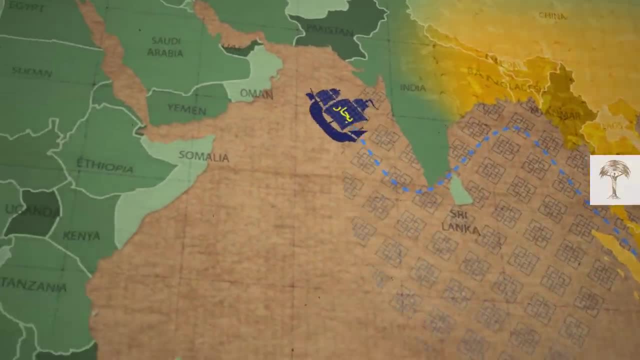 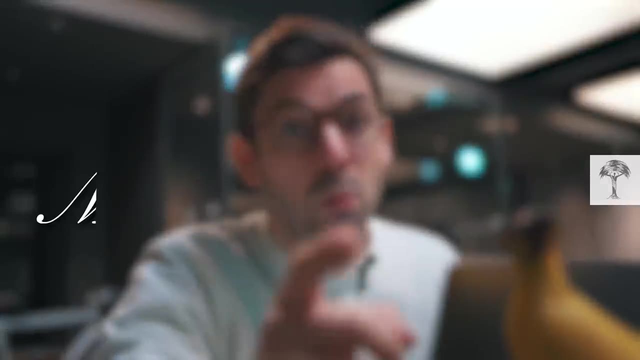 The banana reached Africa with an already very limited gene pool. It was brought there by Arab traders in the 1200s and then became an integral part of the Central African diet. Fun fact, the scientific word Musa originates from Arabic, where the fruit is called Mavus. 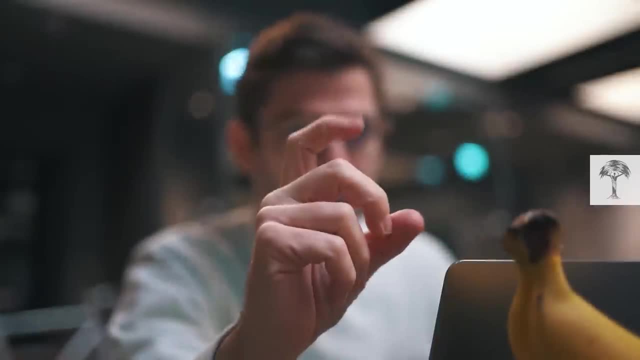 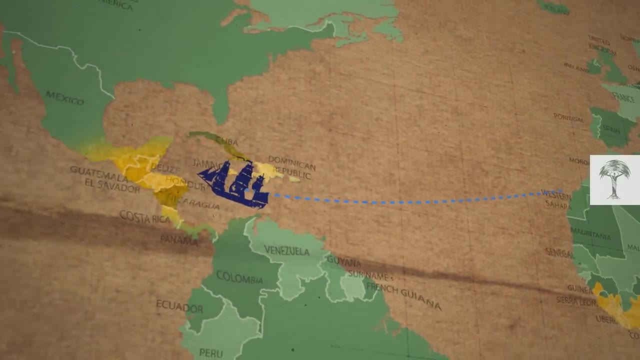 and our name. banana or banan, is a word that means banana. It means finger in Arabic. Anyway, Africa is where Europeans eventually encountered the fruit, And they did what they do best. They took it across the Atlantic and exploited it to the max. 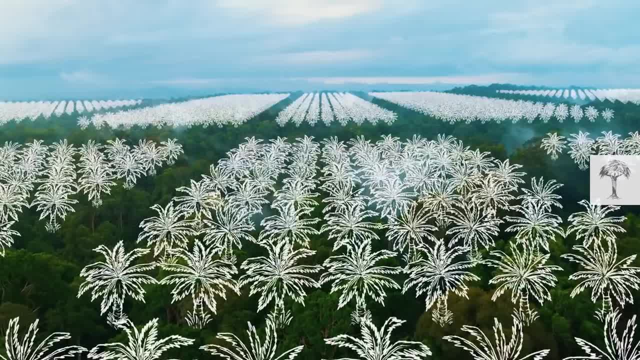 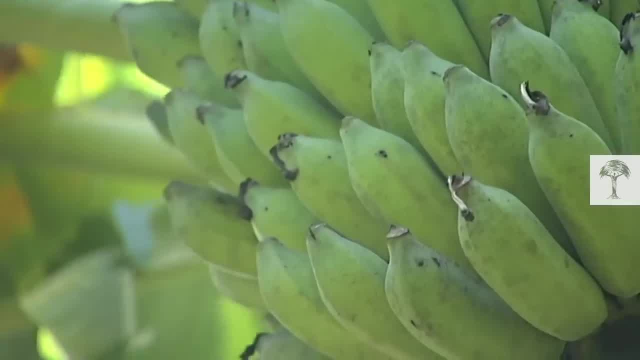 We've wiped out former Central and South American rainforests and paved them with endless miles of banana plantations, All of them planted with one single, genetically identical infertile crop, the so-called Gros Michel, and then its replacement, the Cavendish. 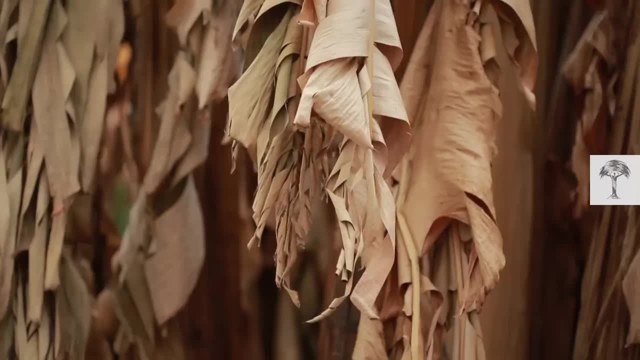 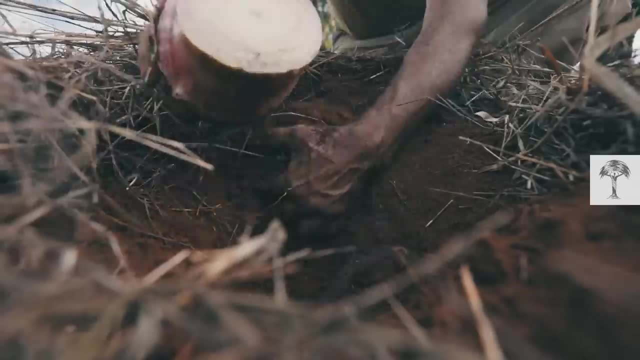 This left the fruit totally defenseless against possible diseases or clots. Yes, the Cavendish banana is in fact infertile. It has no seeds. The way it works is that its corns beget new ones, and then they are taken out and planted. 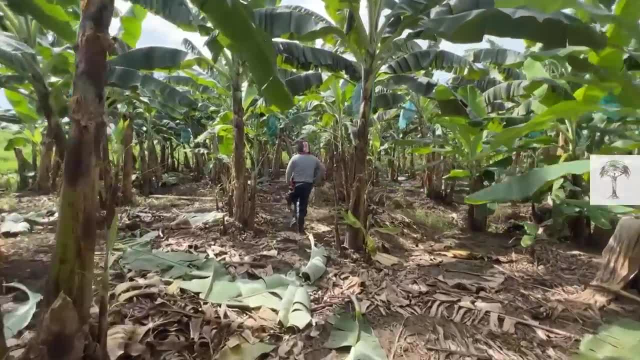 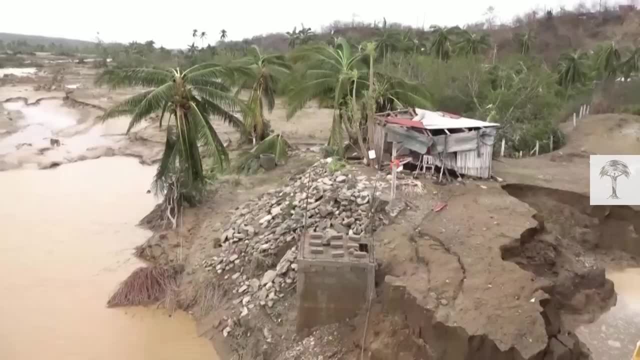 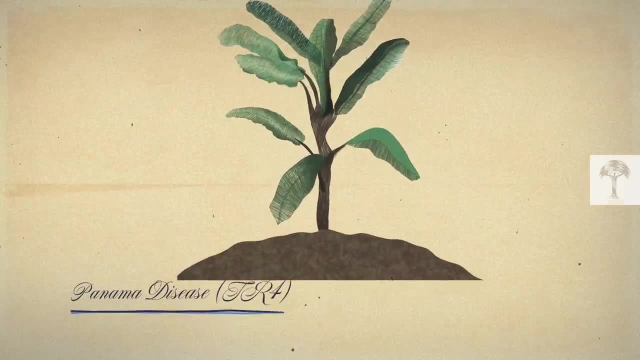 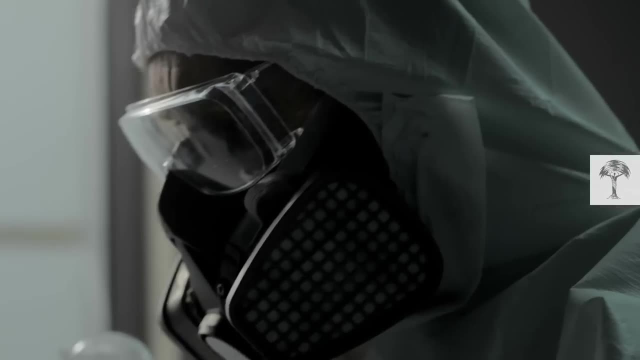 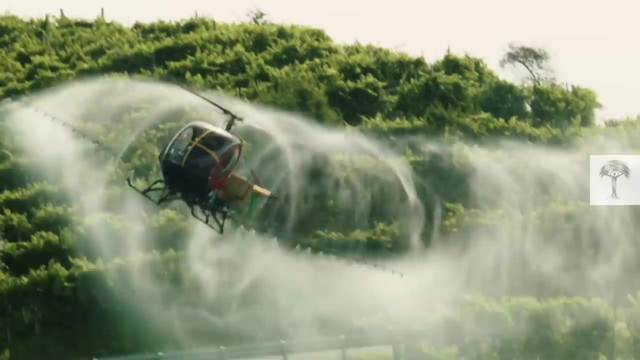 Among others. two diseases are of major concern for the banana farmers: the Panama disease and the Black Sigatoka. Both fungi- One is incurable and can only be contained through literal quarantine, while the other can only be managed with heavy use of pesticides: a chemical blitzkrieg that harms or kills. 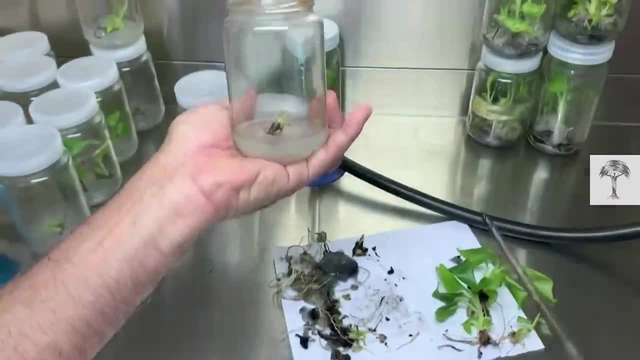 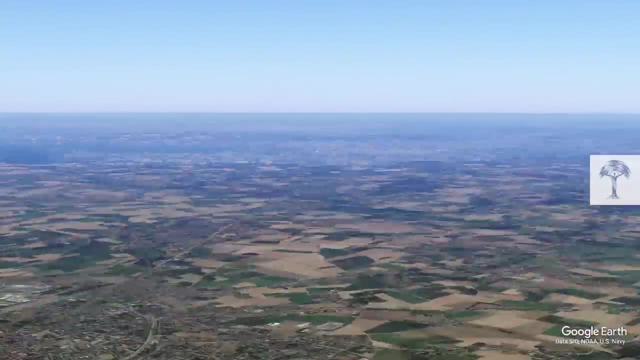 almost everything around it. So what we need is to find or breed a more resistant banana type, or many of them, And it turns out that the world's largest banana collection is only a train ride away from where I live at the Laboratory of Tropical Crop Improvement at the Delft University in 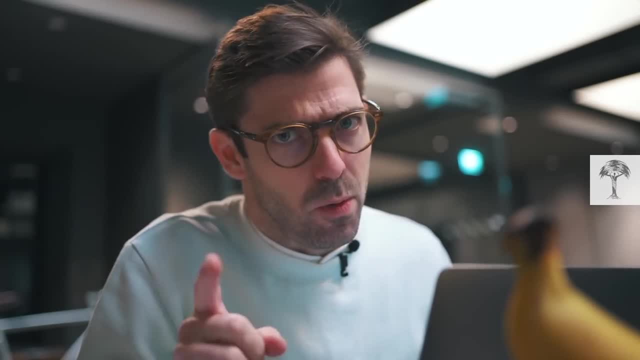 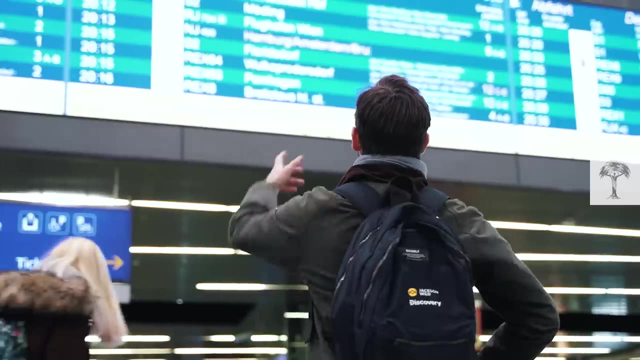 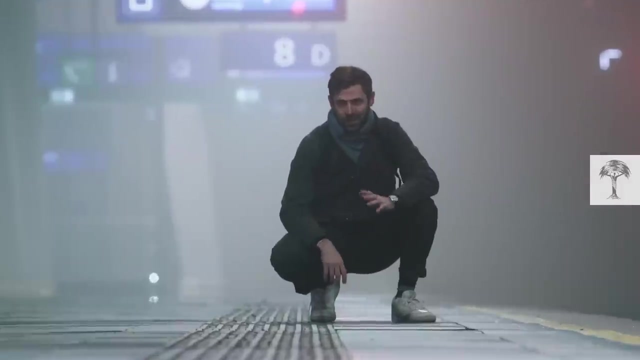 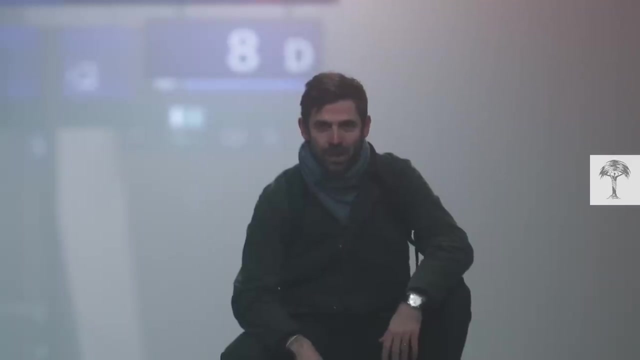 Belgium, And if anyone can tell me how this can be achieved, it will be them. So let's go and find out. Alright, so it looks like going there is much harder than I thought. Austrian railway is striking tomorrow and my train is the first to be cancelled. 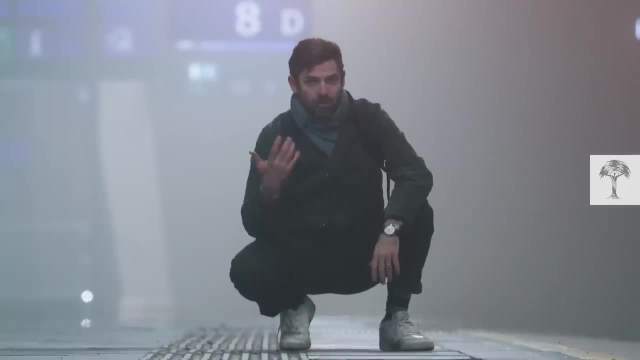 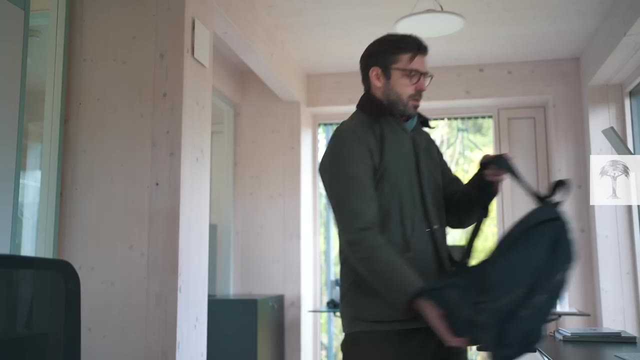 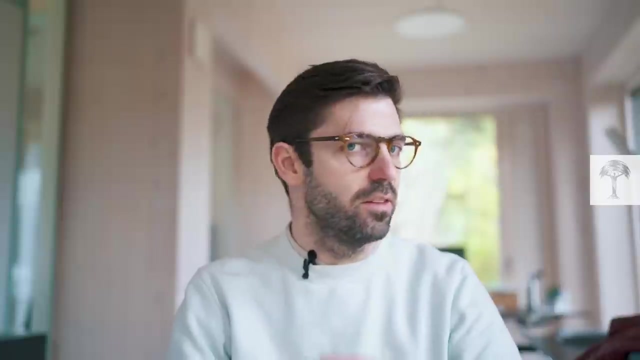 I'm not going to Belgium tonight. I don't know when or if I will be going to the lab. I'll call the guys tomorrow. Let's see where it goes from there. See, the banana is the land breeder's nightmare. It's little to non-existent fertility, and the seedlessness makes it almost impossible. 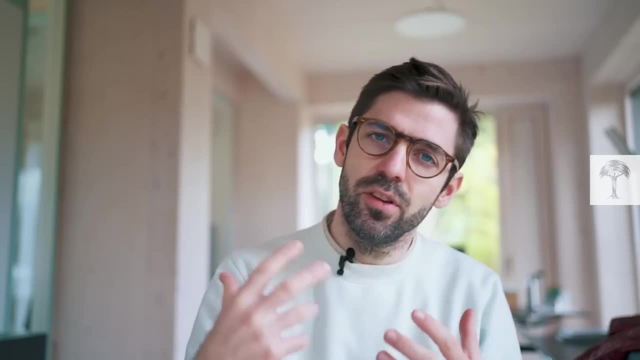 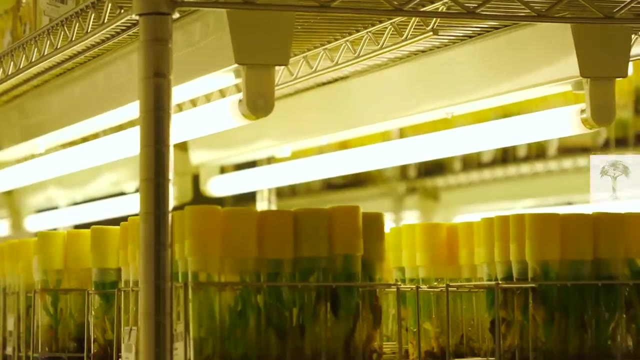 to crossbreed new varieties, And if one of its wild counterparts is resistant to a particular disease, it's still functionally useless if it's susceptible to another malady, And in the lab in Leuven they have more than 1,500 different types of bananas. 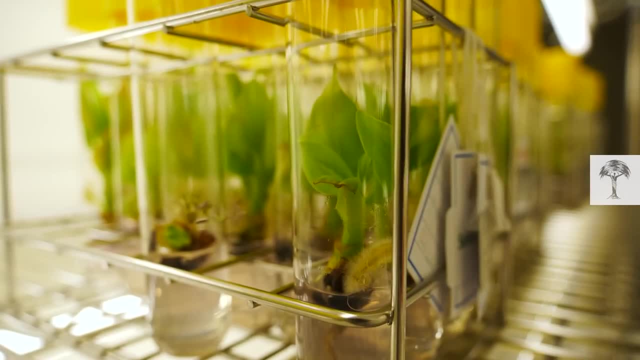 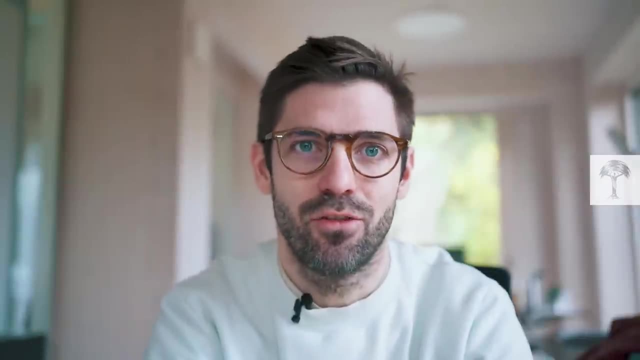 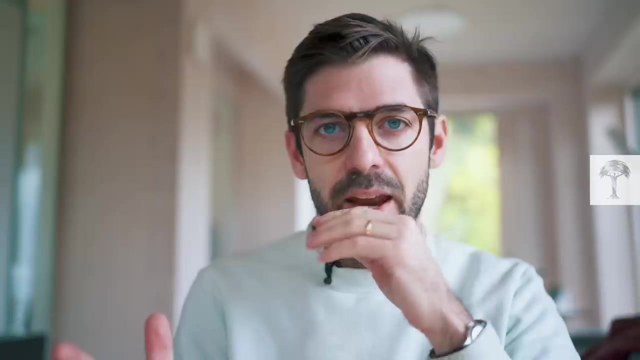 So the traits and features that the banana needs to be used To be fit for the future are to be found there. So I want to find out how these traits can be brought together and make our banana stronger. So I managed to find someone in Belgium who can go and film the lab. 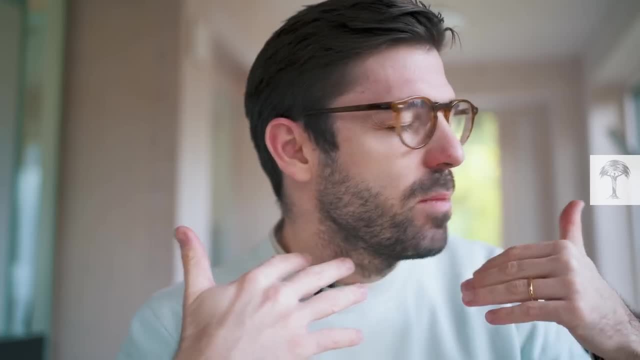 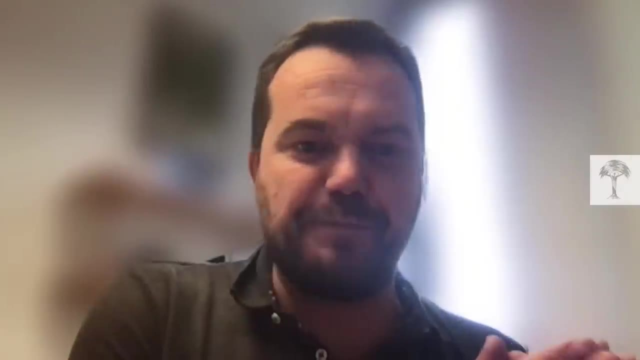 And in the meanwhile I will call the lab leader who can explain this to me much more in depth. Put on my camera. Okay, The Cavendish bananas are triploid, so it means that genetically it's a dead end. There is nothing you can do. 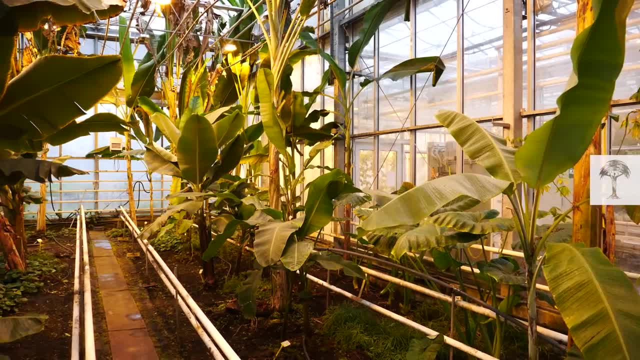 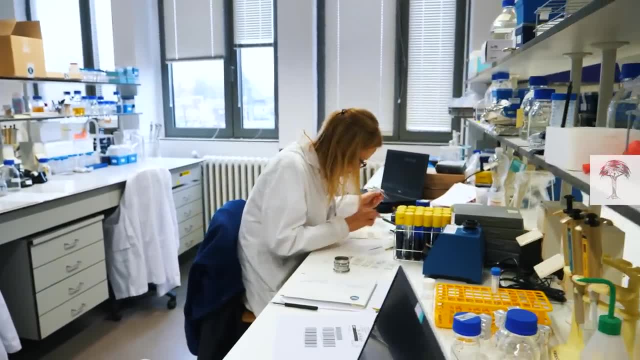 So the only way you could do it is to plant them. There is nothing you can do. All you can do is to go back into the parental lines and to breed again. Of course, novel molecular tools are quite attractive because it means that you can still 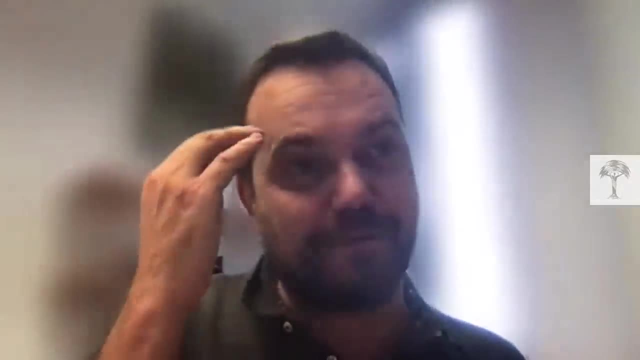 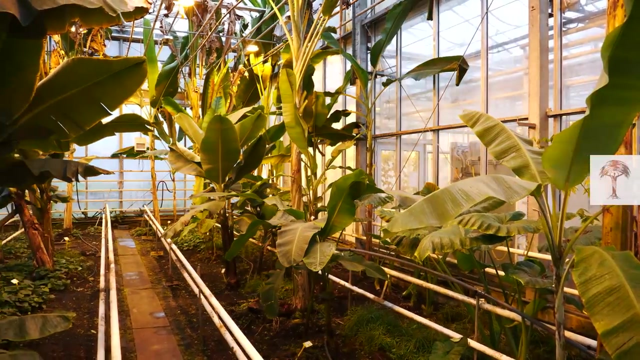 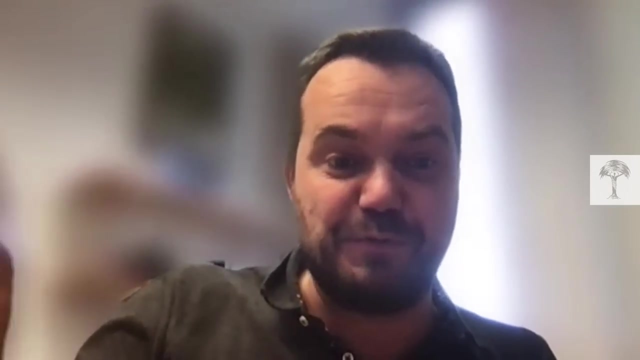 take advantage of the diversity. And now you don't need to think about a very complicated and very tedious and long-term perspective breeding program to breed this gene back into the Cavendish, But you can think of using advanced molecular tools to bring directly the mutation in this. 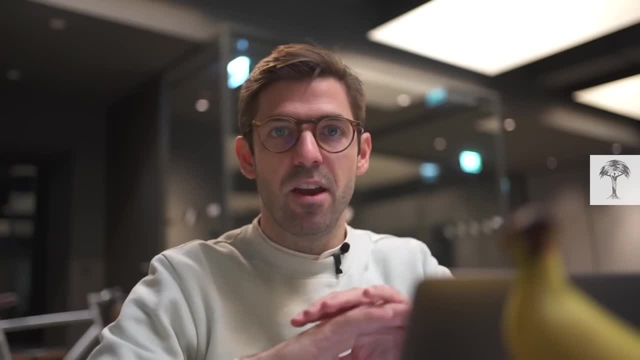 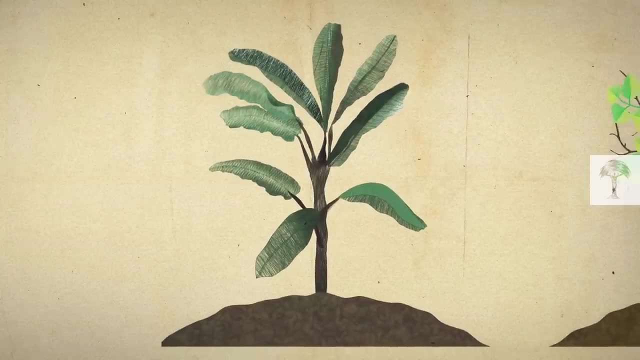 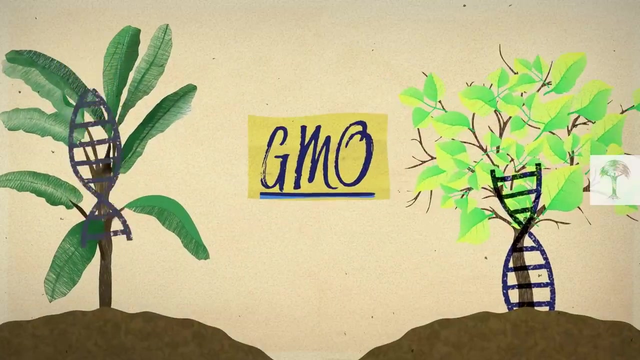 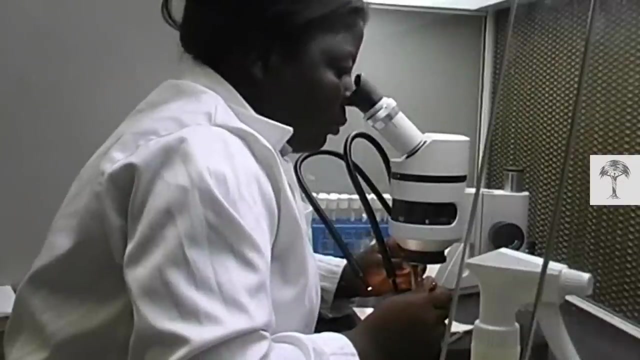 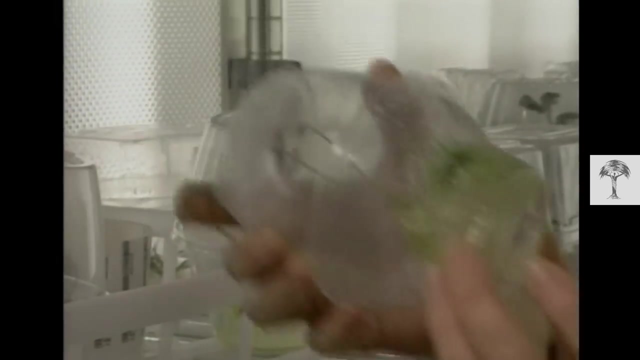 crop species, And that's what we're going to talk about today. So let's get started. The first gene transfer was successfully made in the 1970s and 80s, but methods back then were tedious and imprecise Until. 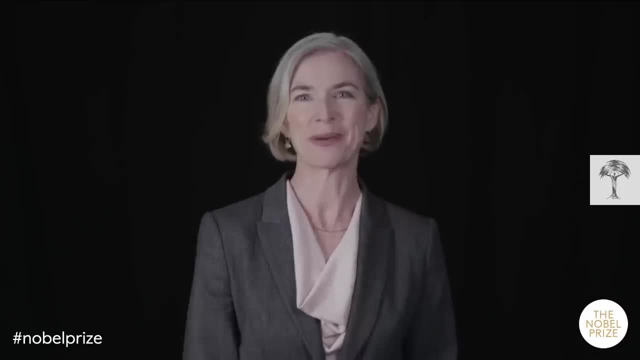 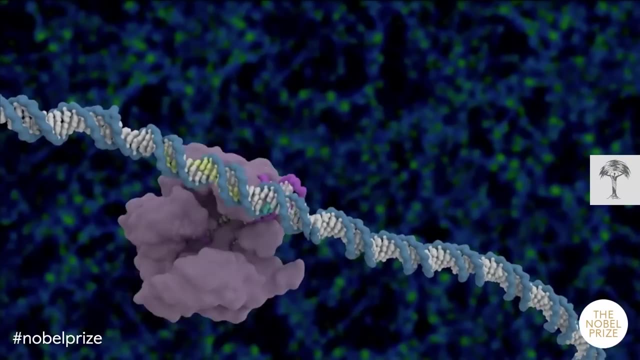 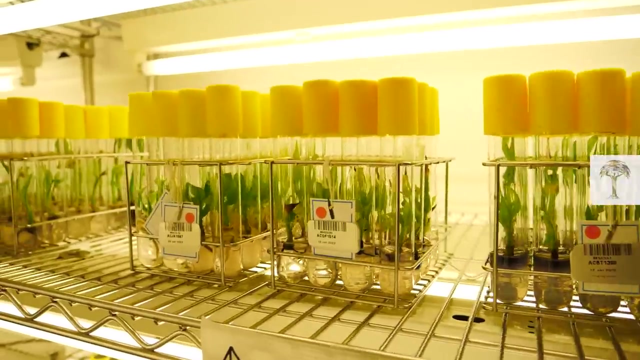 The Nobel Prize for Chemistry. American molecular biologist, Jennifer Doudna, and her French colleague, Emmanuelle Charpentier, discovered the CRISPR-Cas technology: Genetic scissors that can transfer genetic traits with unprecedented speed and incredible precision. Where plant research and agricultural discovery of CRISPR-Cas is a boon, What took months or years through conventional breeding can be obtained through genetic transformation in just days. We realized: okay, now we can take full advantage of the genetic process. We can take full advantage of the genetic process. We can take full advantage of the genetic process. 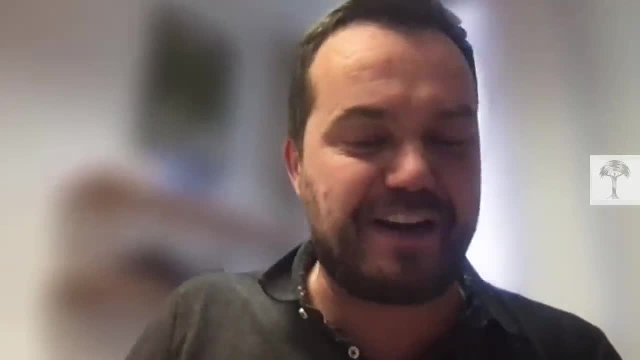 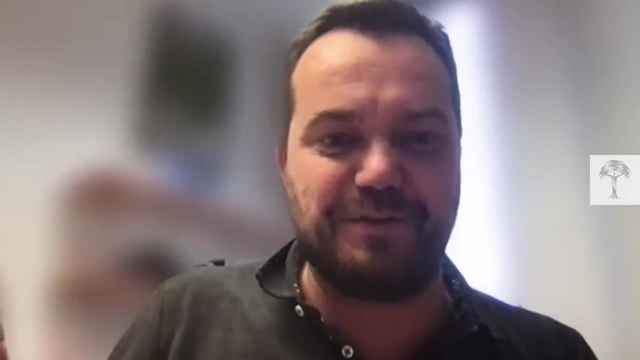 We can take full advantage of the genetic diversity And we are able, with the CRISPR-Cas approach, to mutate precisely in the genome, bring this mutation without any other changes in the genome. Tomato and strawberry varieties resistant to mildew have already been produced, and 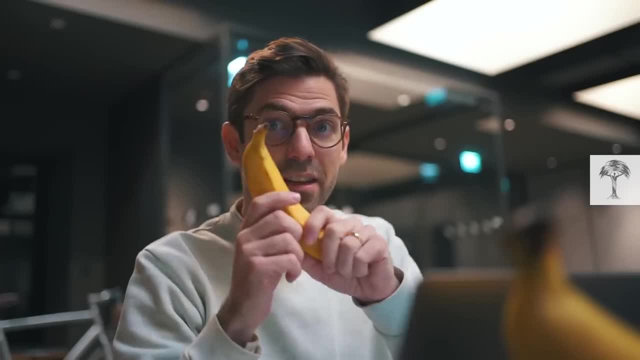 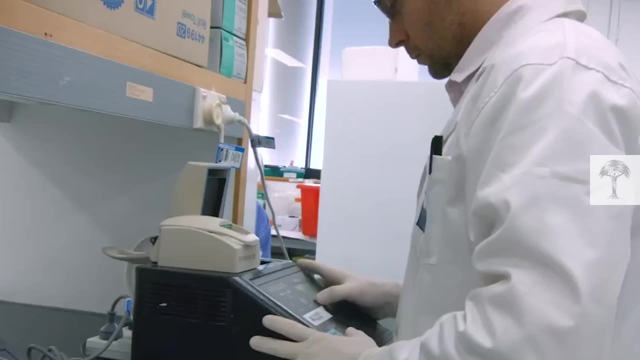 gluten-free wheat is just around the corner, And now it's the Cavendish banana's turn. James Dale, an Australian biotechnologist at Queensland University, and his team have focused on altering Cavendish plants. How There's a new gene from the wild banana, Musa combinata malacensis. that confronts resistance. 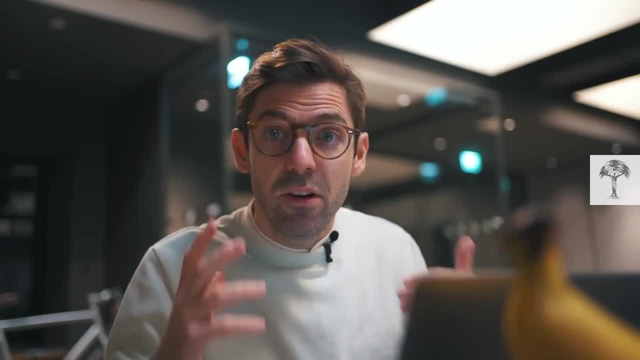 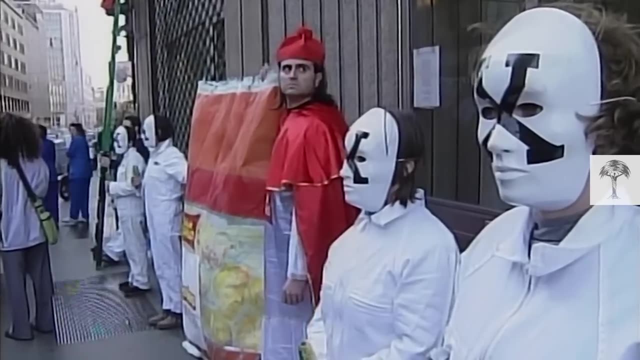 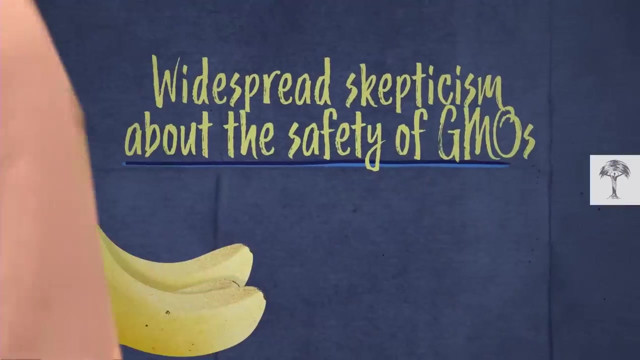 to Panama disease with success. The newly developed variety appears to be immune. These bananas are resistant, But there's a catch, As always. a large number of consumers are skeptical about the idea of genetically manipulated food. According to a survey conducted in the UK, 80% of shoppers wouldn't buy a banana like 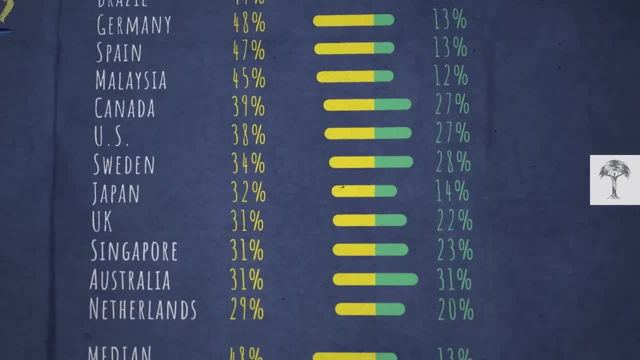 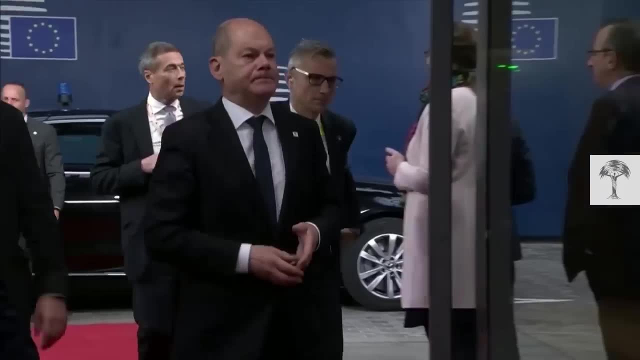 that, On a global scale, a median of 48% find GM food unsafe to eat, with only 13% considering it. People are scared. And then there's the EU. While GMOs are completely normal by now, in the US, they're almost completely banned. 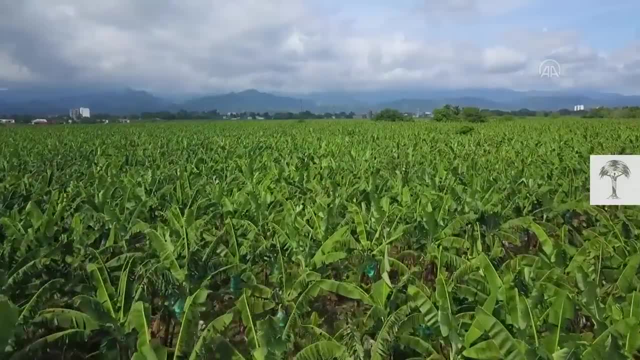 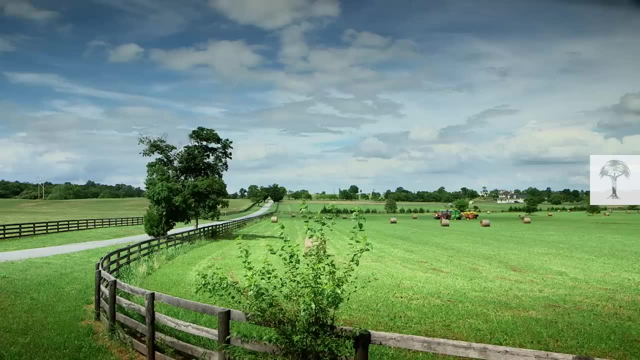 in Europe. But what's often overlooked is that conventional breeding is also a form of genetic manipulation. There's nothing natural about the infertile Cavendish banana. In fact, many of the problems that massive monocultural agriculture has incited can be. 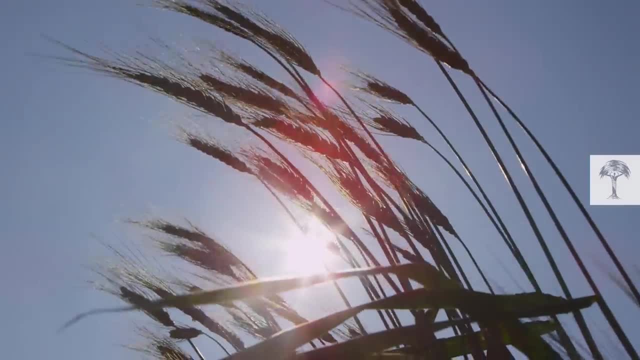 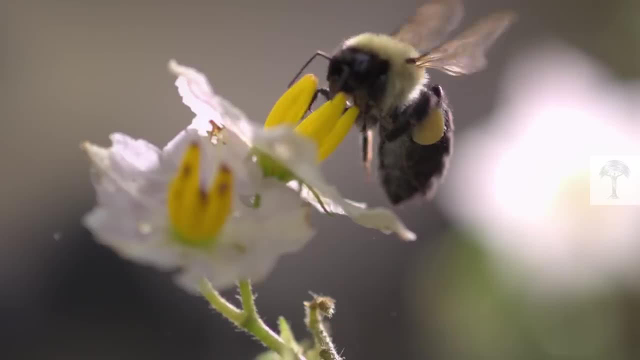 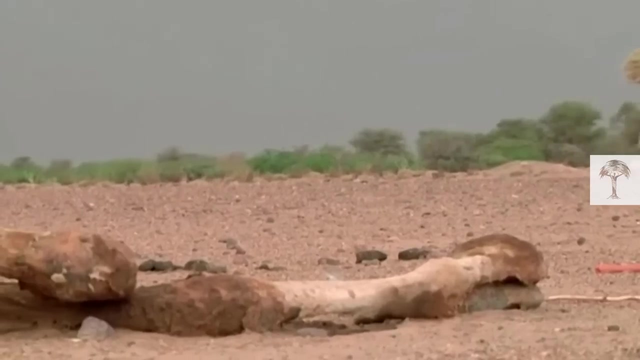 tackled with GM technology. Loss of soil could be reduced through higher yields. Malady resistance could massively reduce pest control, And that's what we're going to talk about today. And, last but not least, hunger. catastrophes provoked by climate-induced droughts could 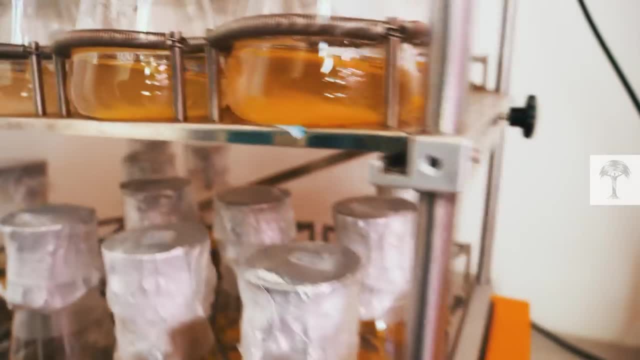 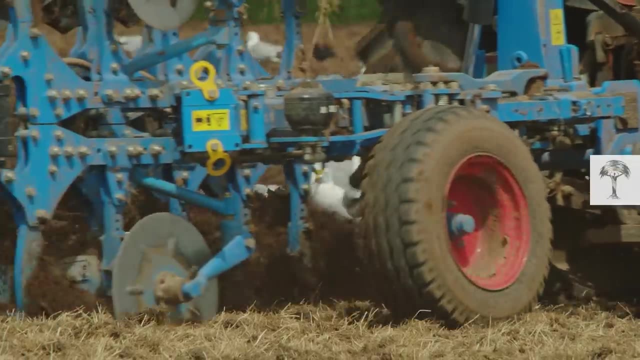 be fought with stronger crops. Yes, there is still this argument that the technology is so young that we still don't have enough experience, that we don't really know what we're doing. and once a crop is out there, you can't take it back. 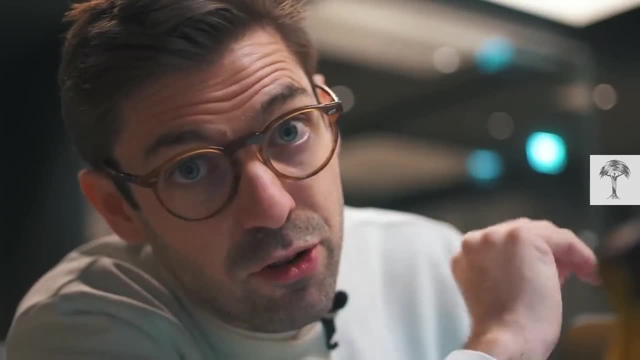 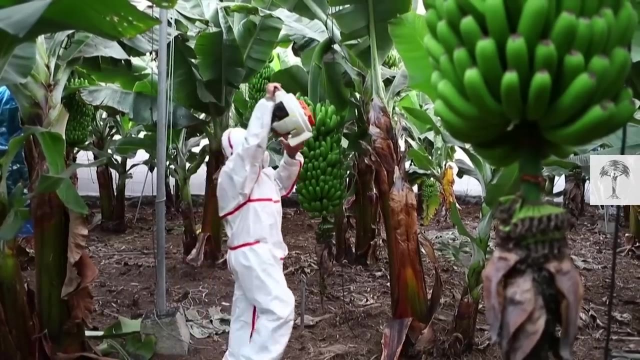 And, of course, plants like these, as is also the case with conventionally bred varieties, need to be tested for humusness before being used in agriculture, And that's what we're going to talk about today. But with current developments, there's not much time left and a seedless banana really. 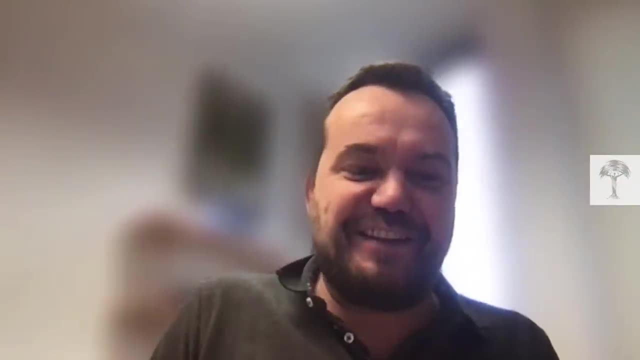 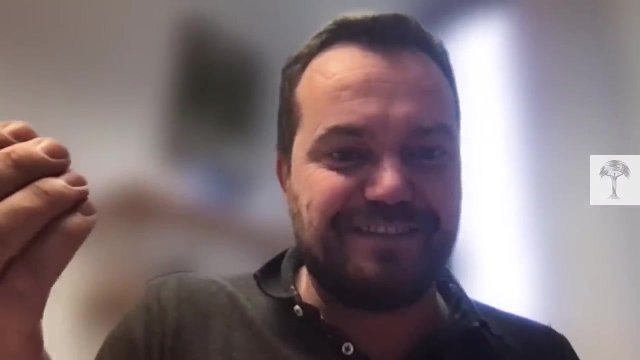 doesn't pose the threat of spreading uncontrolled. I'm not saying this is the only response to the challenge we are facing. That would be again a mistake to say so- or at least we have to test the potential. We cannot go away from this without testing it right.